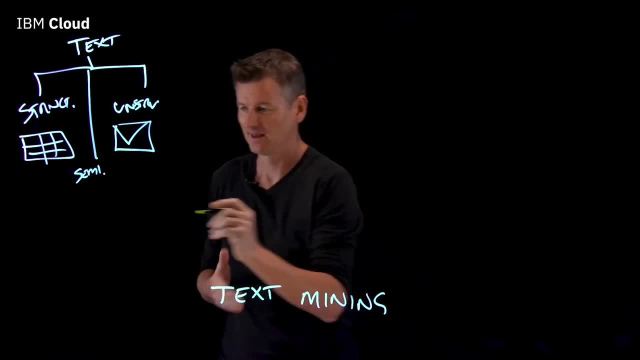 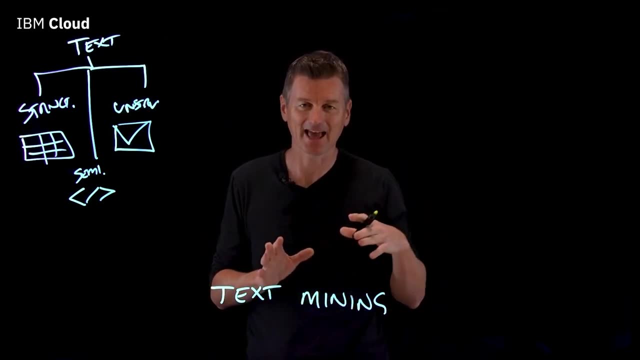 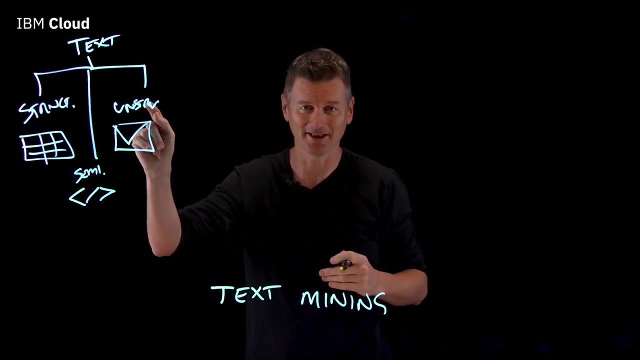 to meet the requirements of a relational database, So think of like XML or JSON or something along those terms. Now it turns out that something like 80% of the data in the world resides in an unstructured format, So there's plenty of opportunity to put text mining to work. 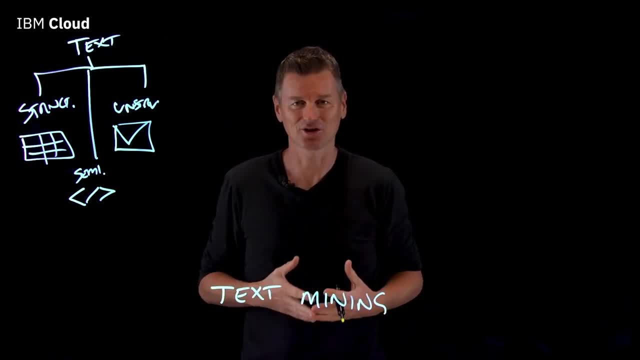 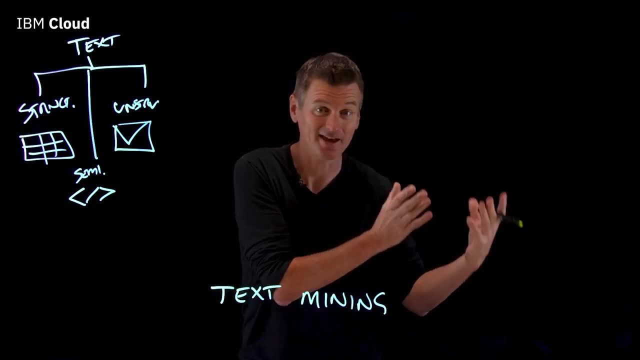 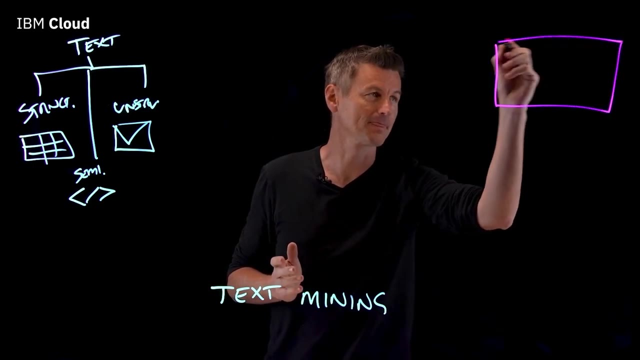 We use text mining to generate an index of structured concepts to be able to answer questions like which concepts occur together and what do the concepts predict. To do this, we'll go through four different stages. Okay, so stage one, That is, identify. 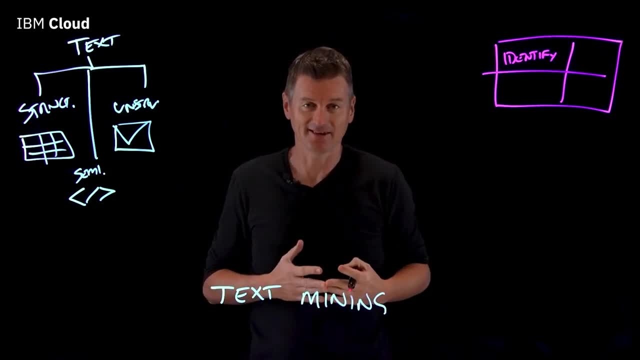 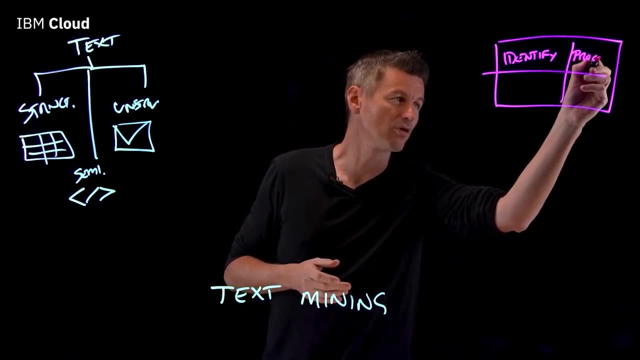 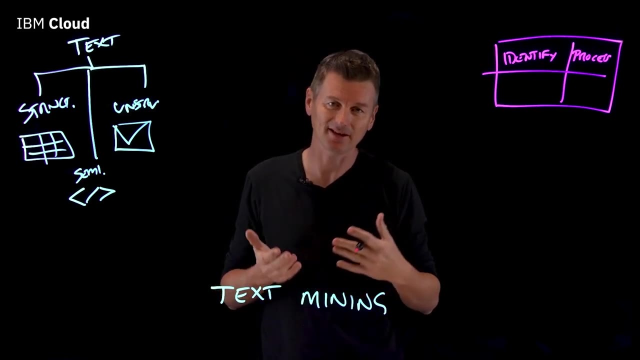 This is where we identify the text that is to be mined, And that might be a collection of news articles or product reviews. In stage two, we process the text to remove noise and to standardise the format, So this includes doing things like removing stop words, tokenising the words. 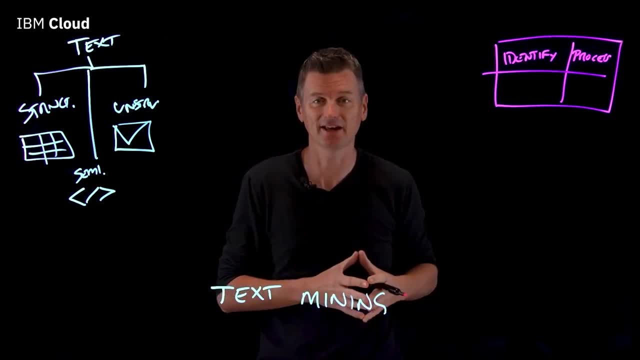 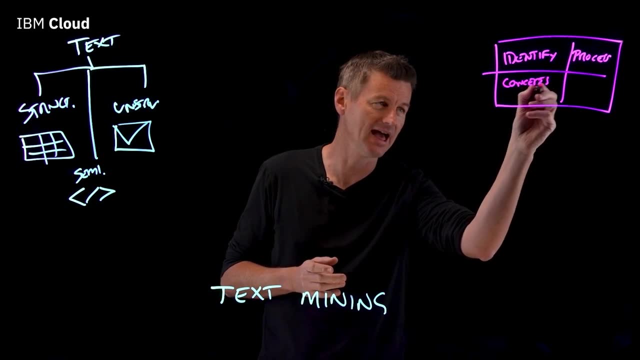 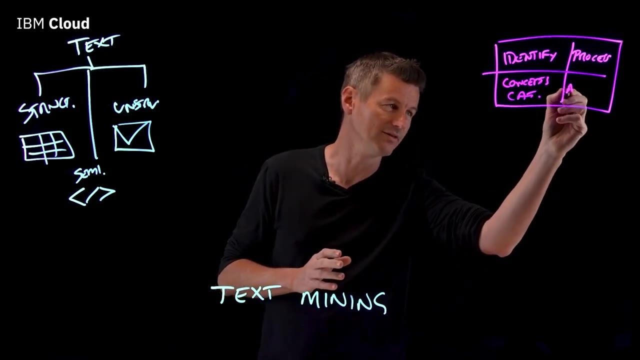 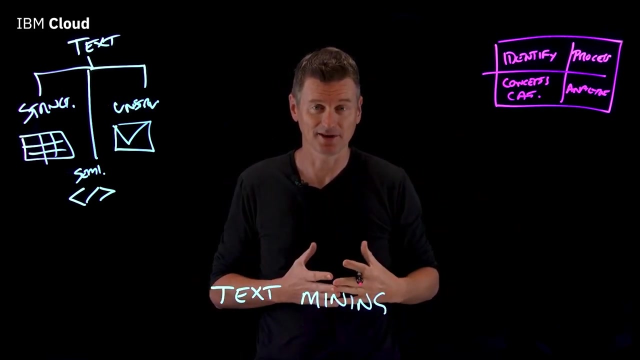 lemmatising and part of speech tagging- All sort of things like that- are used in the processing stage. Then stage three builds the concept and the categories, And then in stage four, we analyse all of this to really make predictions and to discover relationships. Now, first of all, let's focus here. 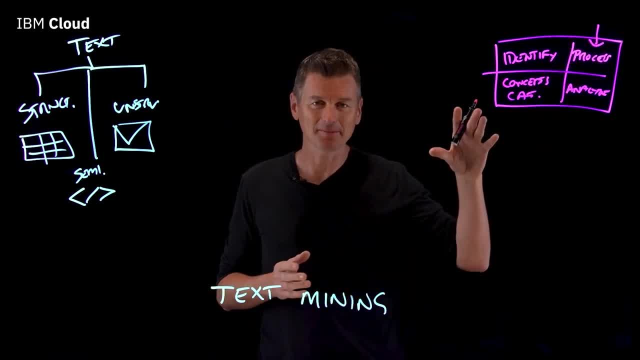 on stage two for a moment Now. first of all, let's focus here on stage two for a moment now. first of all, let's focus here on stage two for a moment. The primary problem with the management of all this institutional text and data is that there. 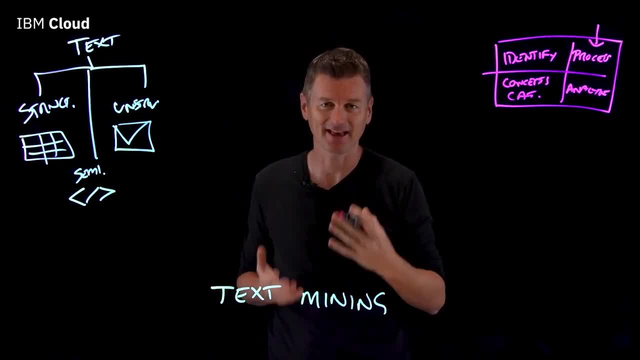 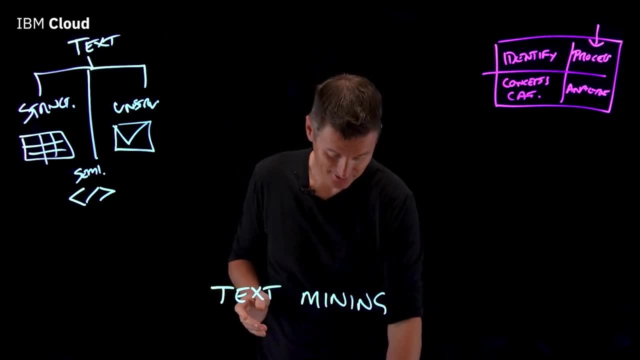 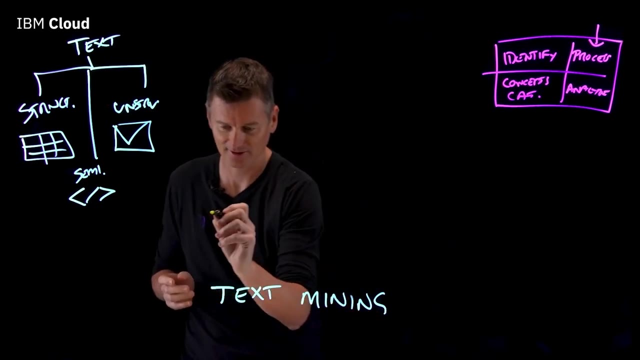 are no standard rules for writing text so that a computer can understand it, But language and consequently the meaning varies for every document and every piece of text. So if we take a phrase, let's say reproduction- That pen's not so good, Let's try this one: Reproduction. 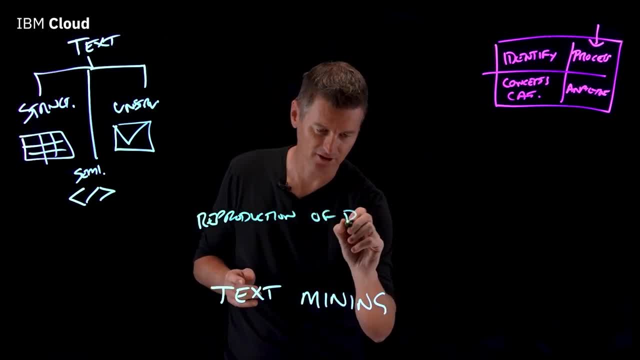 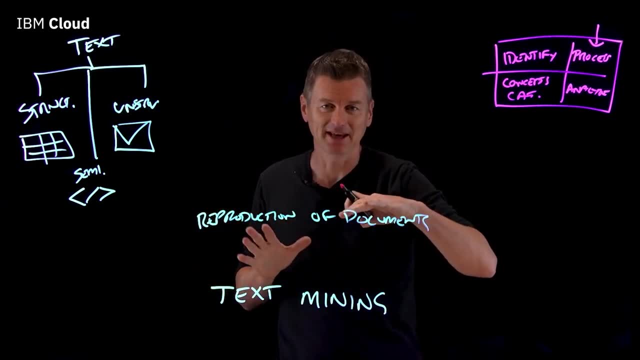 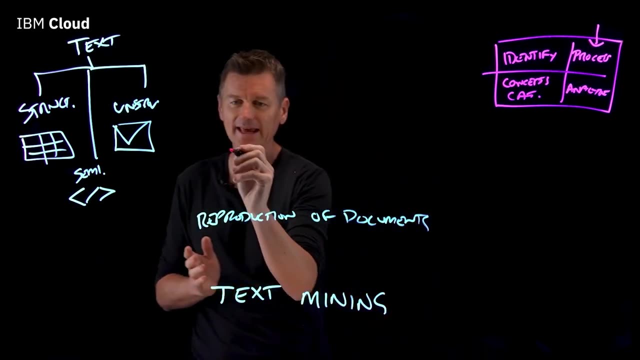 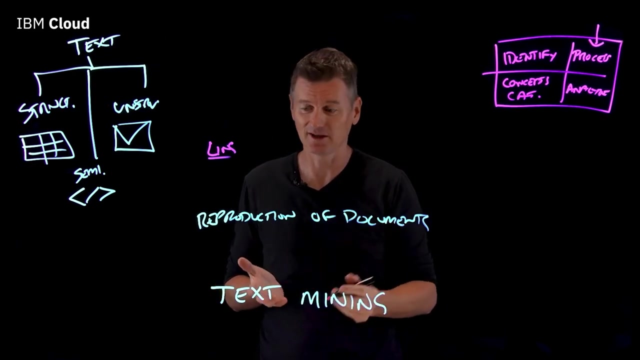 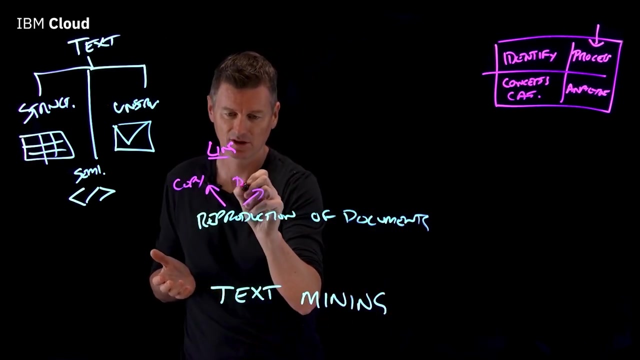 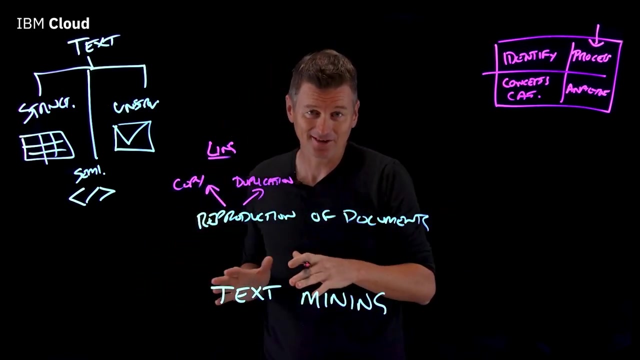 of documents. How can we expand the meaning of this? What other words would be cinnamons for reproduction? Well, a linguistics based text mining model might suggest a couple of words for reproduction, like copy. Or it might suggest duplication, and those look good. and that's because linguistics-based text mining 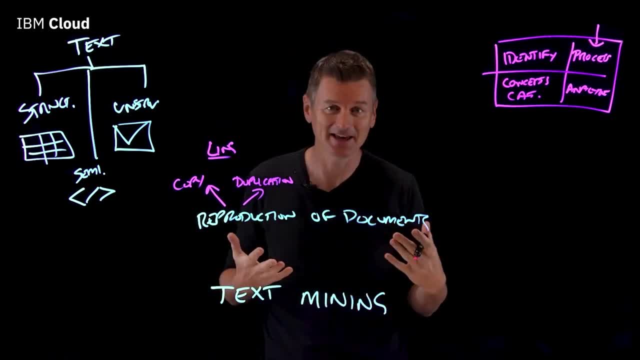 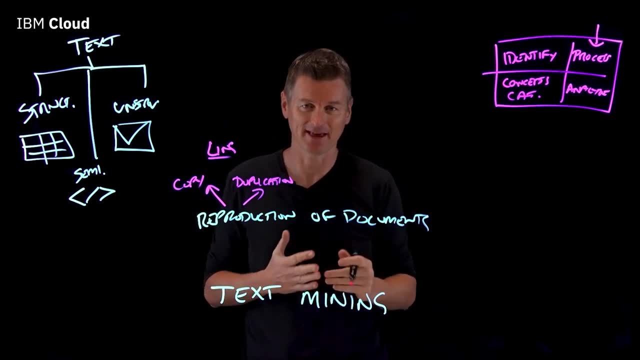 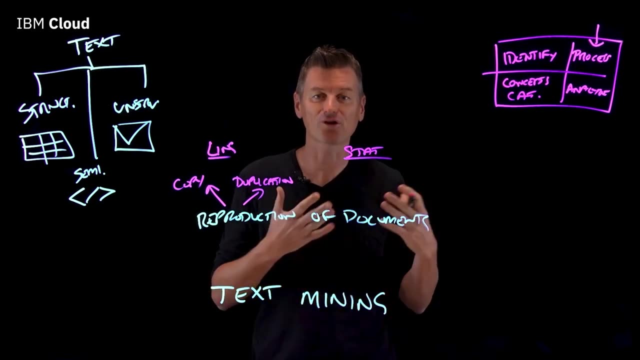 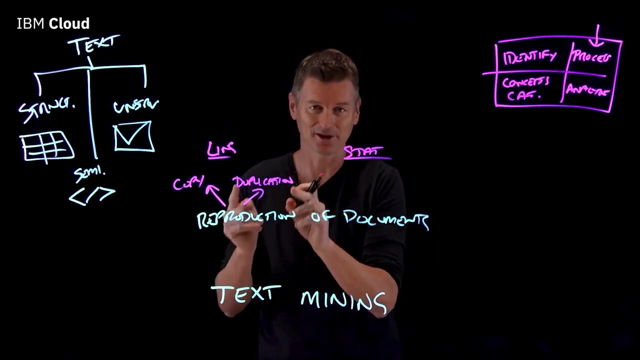 applies the principles of natural language processing, or NLP, to the analysis of words, phrases and syntax of text. An alternative to linguistics-based text mining is statistics-based text mining and that uses calculations of frequency to derive related terms, and statistics-based text mining tells us that reproduction is related to the term. 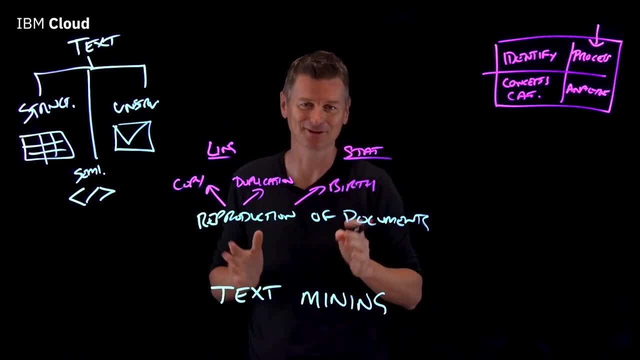 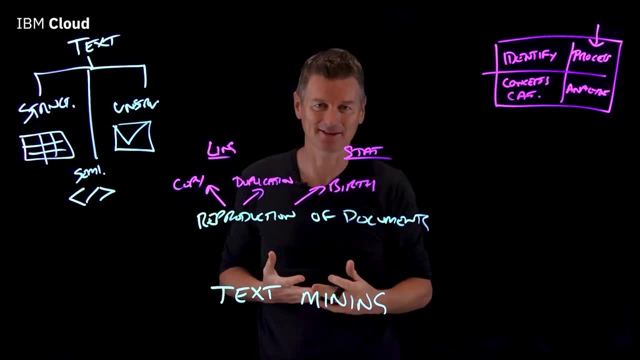 birth. That's going to generate some highly irrelevant results. so using NLP to understand the language used cuts through the ambiguity of text, making linguistics-based text mining the most effective way for solving the number of questions asked- more reliable approach. and it's this processing that brings us to the category building of stage. 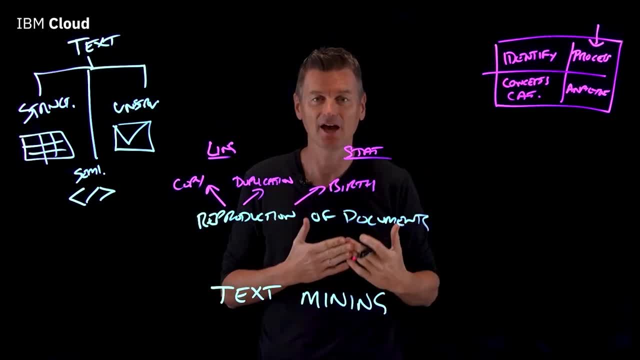 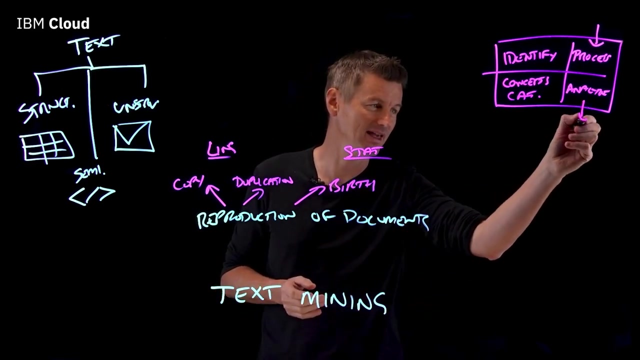 three, where the concepts and the types that were extracted are used as the category building blocks. when the build categories, records and documents then assigned to those categories, we can take a look at the text that they contain and match an element of the categories definition and from there the relationship discovery and the prediction analysis is performed here by data. 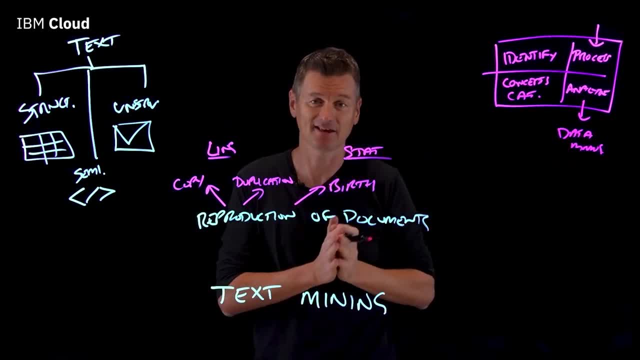 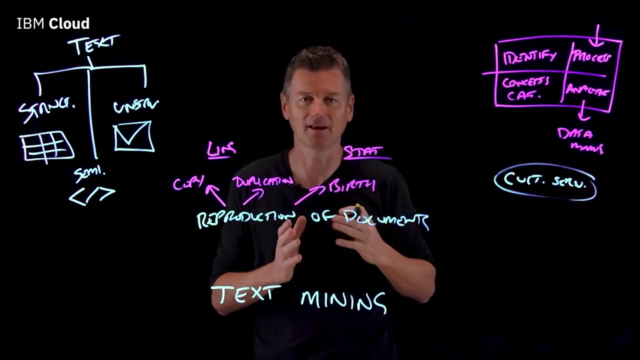 mining and data mining is a topic that we've addressed in another video, so check that out if you want to see some more detail. now, beyond sifting through product reviews, where can text mining also be applied? well, in the wider field of customer service, text mining can be applied to work with sentiment analysis and that can provide a mechanism for